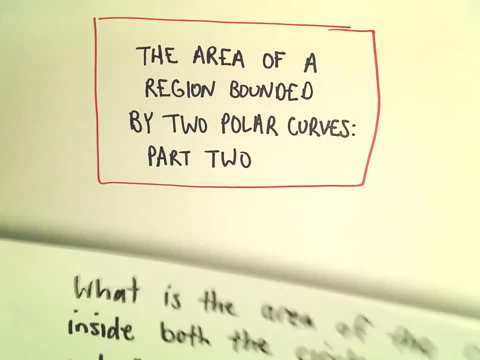 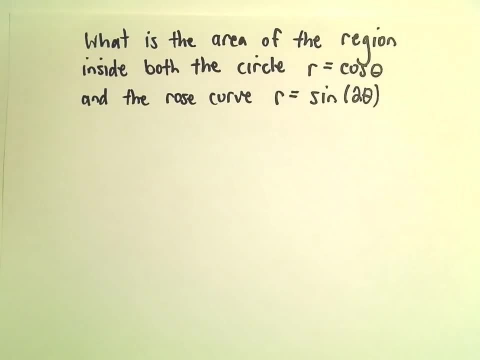 Alright, here we're going to do another example of finding the area of a region bounded by two polar curves. So here we're going to find the area that's inside both the circle- r equals cosine theta and the rose curve- r equals sine 2 theta. 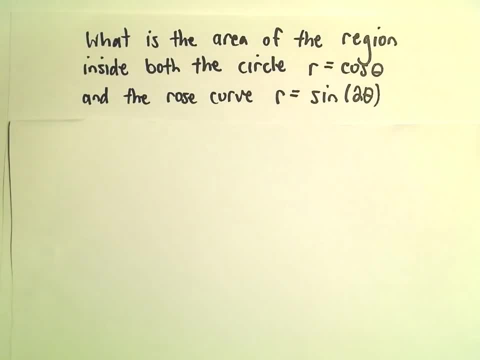 So I'm going to do a quick little sketch of these, hopefully. So the first one here I'm going to graph is going to be: r equals sine of 2 theta. So r equals sine of 2 theta For a rose curve, recall if the number in front of theta is even. 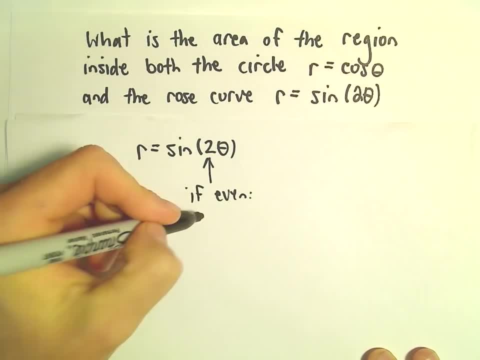 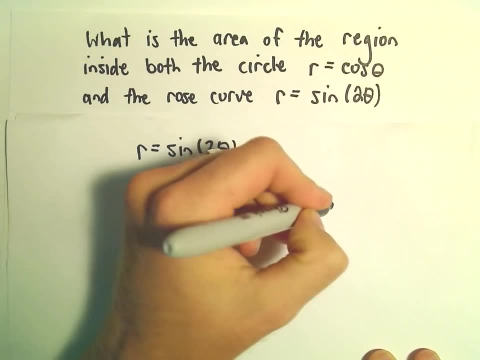 If it's even, which? well, certainly it is in this case. we take 2 and multiply it by whatever that number is. Well, in that case, this is 4.. And that's going to give us the number of petals, The number of petals on our rose curve. 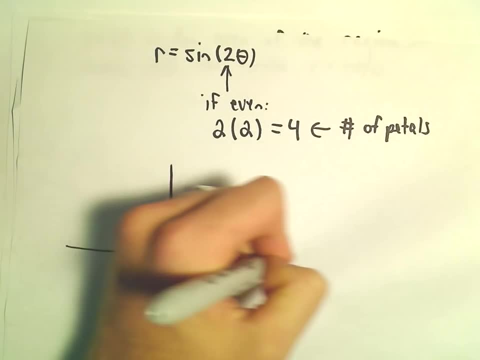 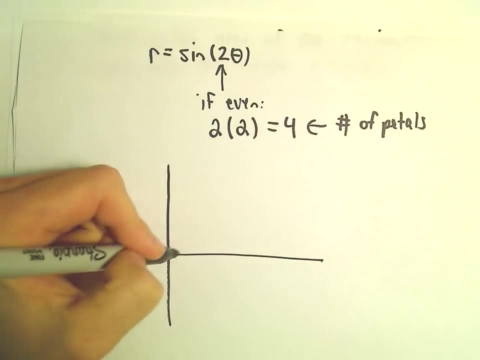 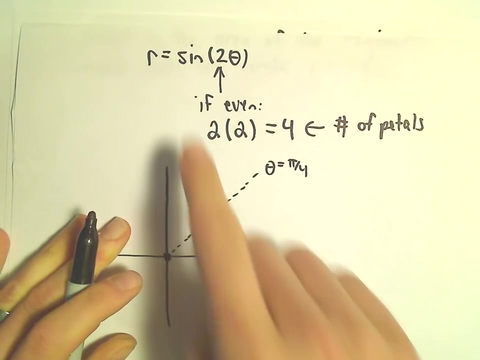 So, Notice, If theta equals 0,, we'll get sine of 0,, which is 0.. Notice that theta equals pi over 4.. We'll get sine of 2 times pi over 4,, which is going to be sine of pi over 2.. 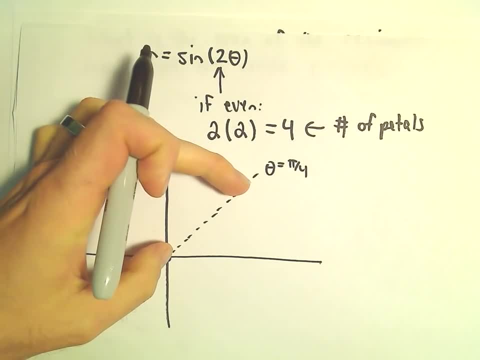 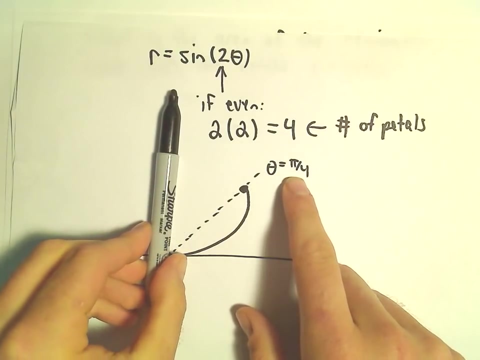 And that's where we're going to get our r value of 1.. Kind of our maximum distance from the origin. And as theta increases from 0 to pi over 4, our r value will increase. And then as theta increases from pi over 4 to pi over 2, we'll get values on the inside from pi over 2 to pi. 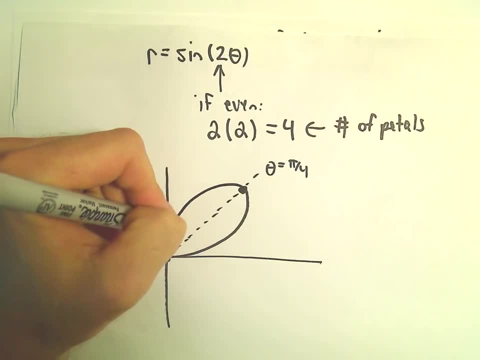 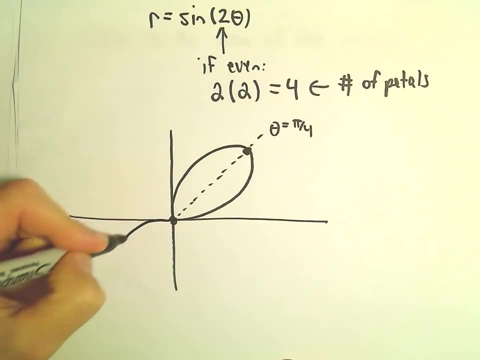 And that's going to make our radius decrease back to 0. And that'll give us one little petal of our rose curve. You could plot some more points and you would find that basically it's just symmetric. We're going to get a petal in each little quadrant. 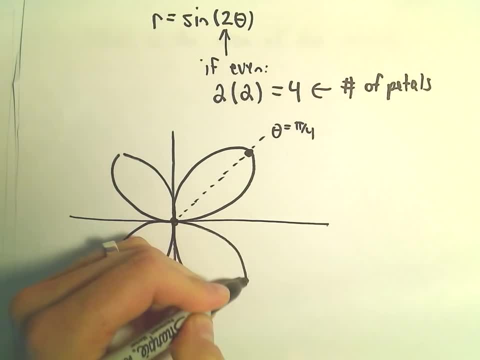 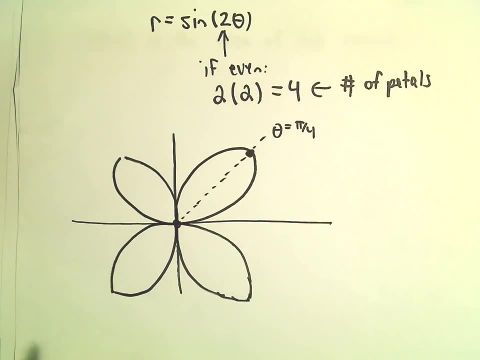 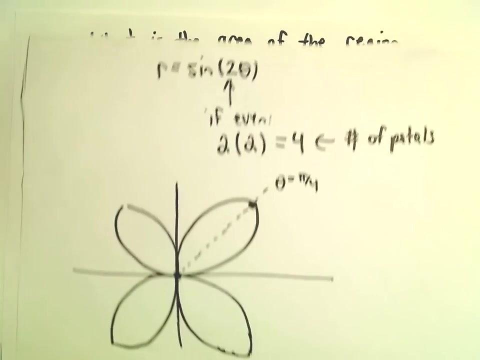 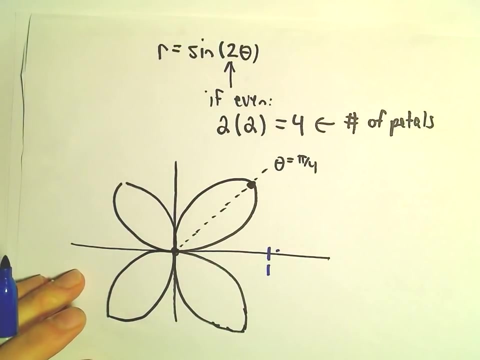 So our rose curve would look something like this: Alright, so there's a very rough sketch of r equals sine 2 theta. R equals cosine theta. So r equals cosine theta is just a circle. It's going to go out to a distance of 1 on the x-axis. 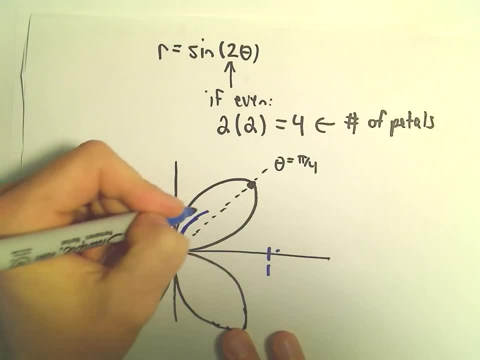 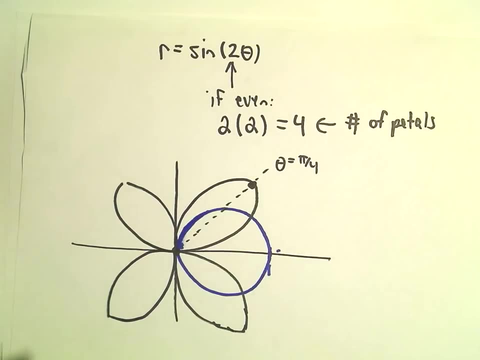 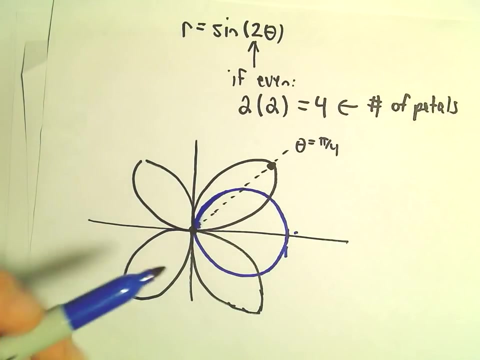 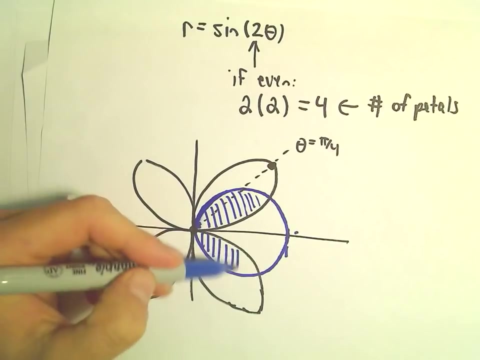 So let's see if I can make a little circle here. Okay, so there's our little circle, Alright. so now what I'm going to try to do again is we're trying to find the area inside of these two circles. So we're trying to find this little area and this little area as well. 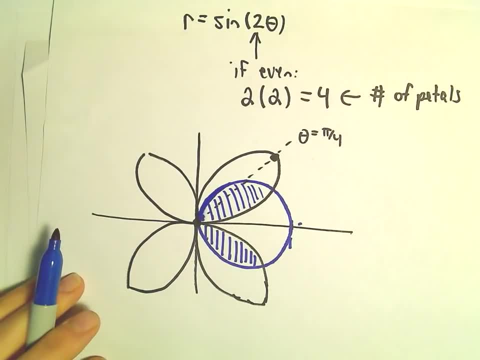 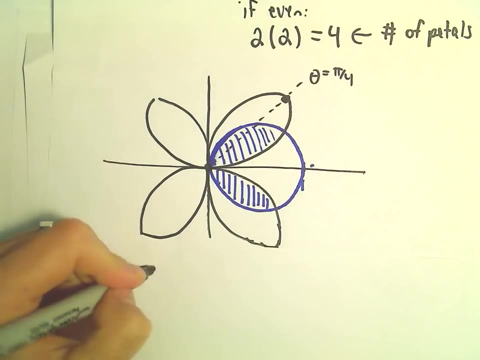 They should be symmetric, just based on the symmetry of our curves. So what I'm going to do is I'm going to find the points of intersection by setting them equal to each other. So let's see, we had r equals sine of 2 theta. 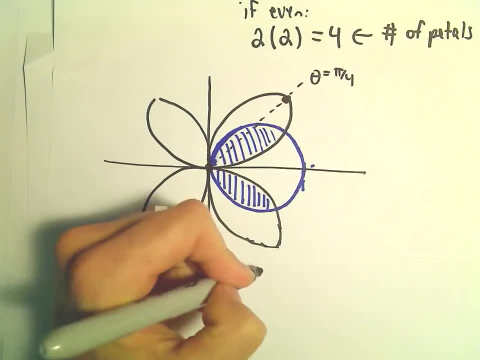 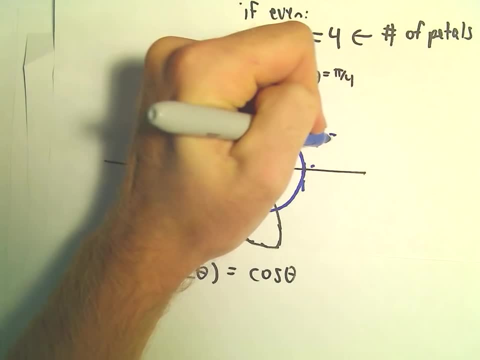 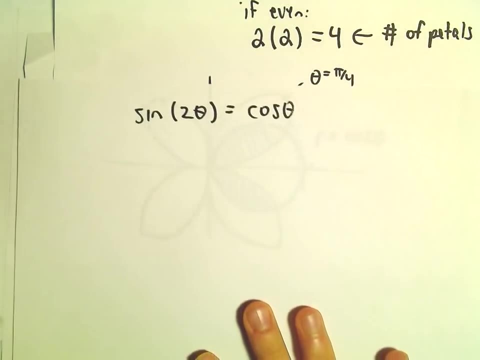 And we had r equals cosine theta. So again, we'll just set those equal. So let me label this one. This is going to be: r equals cosine theta. Well, to find the points of intersection, I'm just going to use a little trig identity. 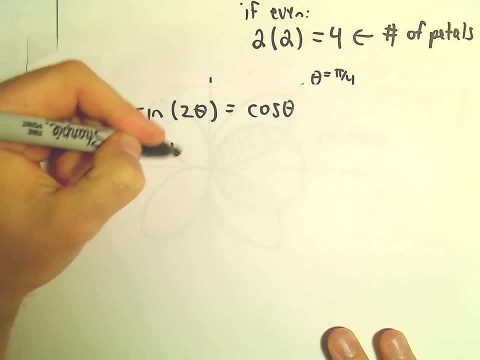 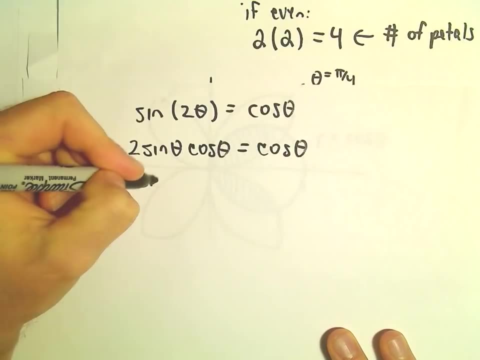 Sine of 2 theta. Well, that's 2 sine theta. times cosine theta equals cosine theta. We can subtract cosine theta from both sides, Factor the cosine theta out, Then we'll be left with 2 times sine theta minus 1 inside of our parentheses. 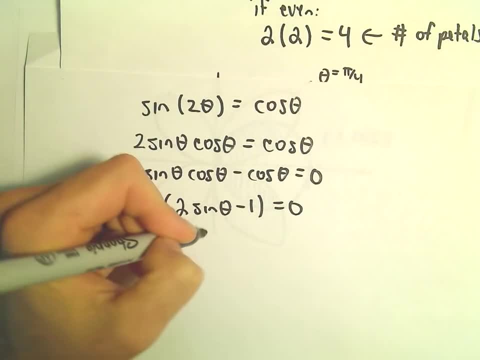 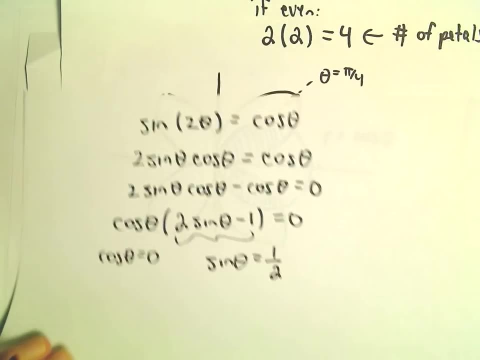 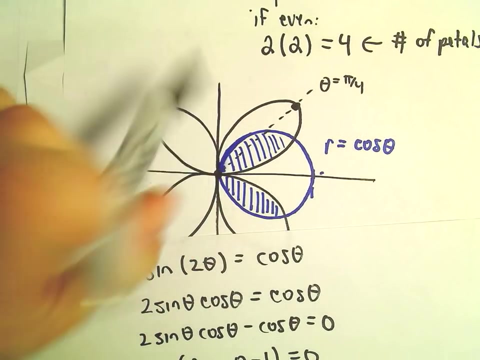 So we'll get: cosine theta has to equal 0. Or from our other factor we'll get that sine of theta has to equal 1, half Well, cosine of theta equals 0 at pi over 2.. So that's definitely going to be one of our little points of intersection at pi over 2.. 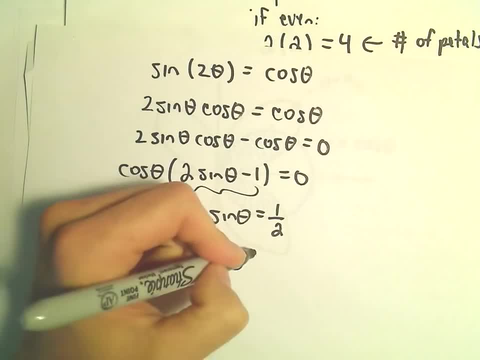 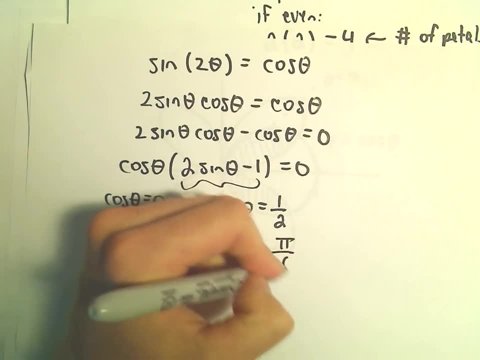 Let's see, sine of theta is going to equal 1 half. I guess one place in the first quadrant where sine of theta equals 1 half is going to be at the angle pi over 6.. And I think, just using these two. 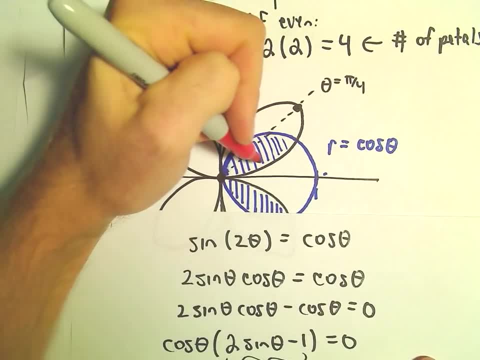 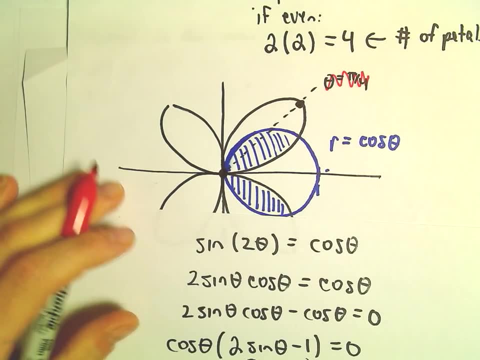 that'll be enough for us to figure out to be able to solve the problem. All right, so forget all about the pi over 4.. We really don't need that anymore. That was just kind of to help us sketch the rose curve. 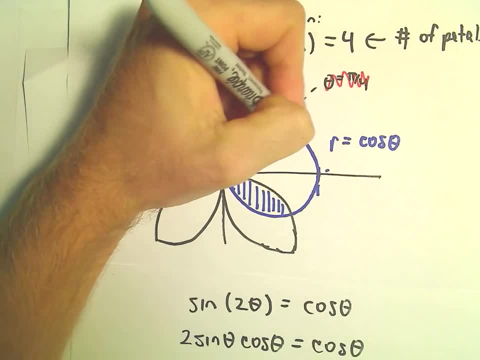 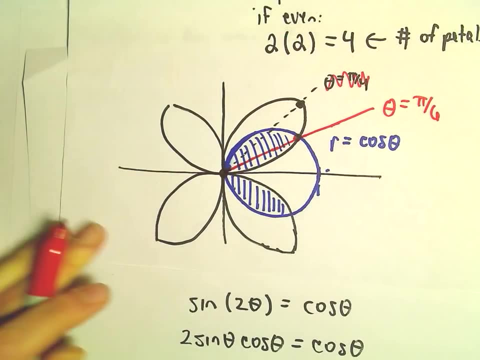 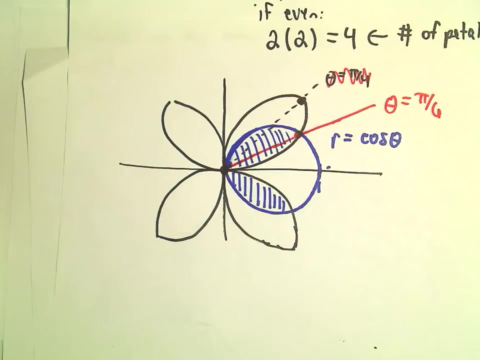 This point of intersection again, where they're crisscrossing. that is going to be useful. That's going to correspond to theta equals pi over 6.. So what I'm going to do to find the actual area now that we're interested in. 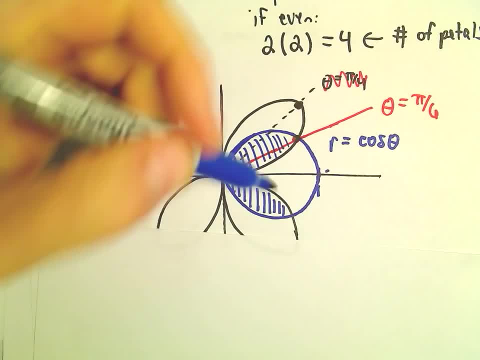 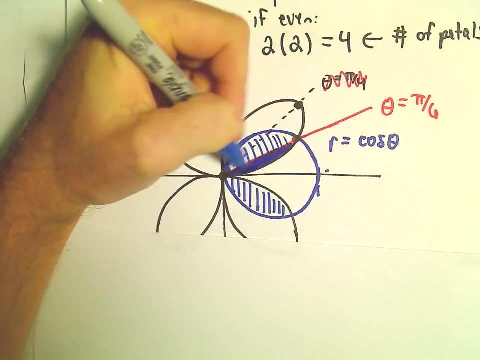 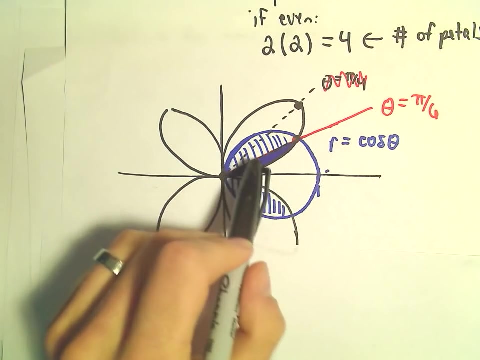 the first thing I'm going to do is set up an integral to find this lower portion that's enclosed. So I'm going to find this darkly shaded region Okay, so to get that very dark, that sort of it's not half. 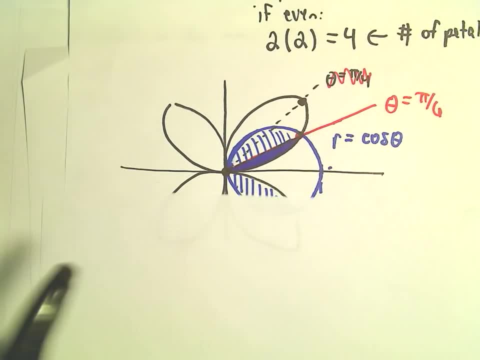 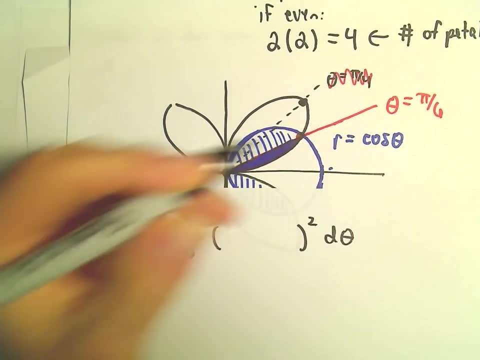 but this bottom part of sort of the top part. what I'm going to do is I'm going to use my formula, So it's going to be 1 half r squared d theta. Okay, so the limits of integration are going to correspond to 0 to pi over 6.. 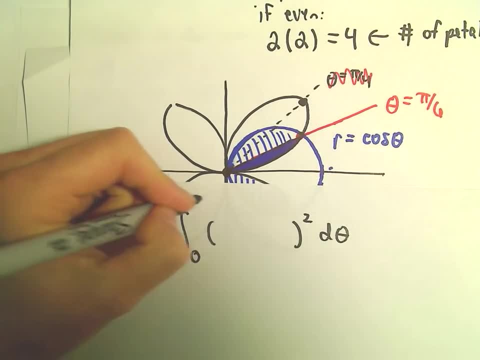 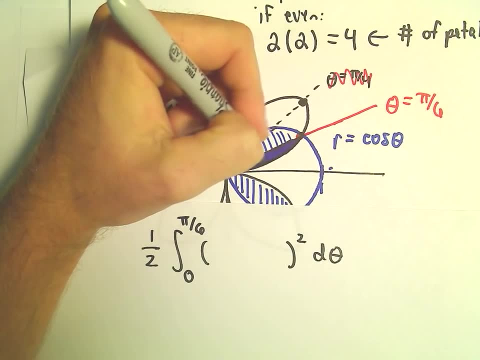 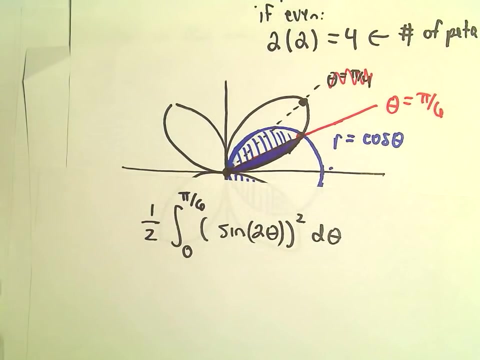 That's what we just found. So 0 to pi over 6.. And notice that the curve that it's bounded by, the curve that it's trapped inside of, that's our rose curve, which was sine of 2 theta. Okay, so that's going to give us this bottom portion. 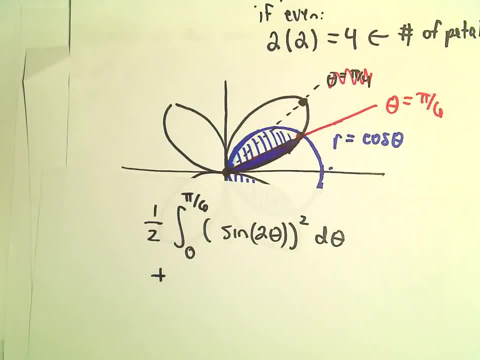 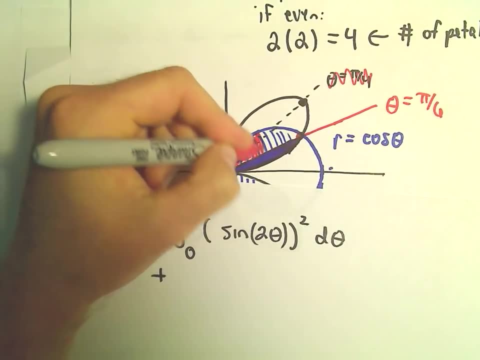 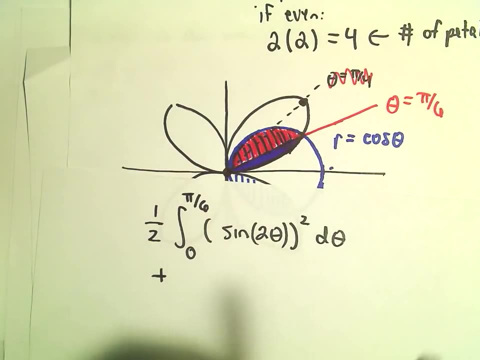 Well, to figure out the top part. okay, so to figure out the top part. well, now I'm going to do the same thing. I'm going to compute another integral, So I'm going to have 1, half the integral. 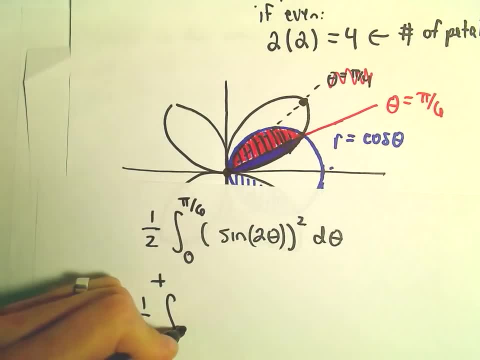 Well, now we start at the angle pi over 6, so that's going to be our lower limit of integration. We're back at at the origin, at theta equals pi over 2.. And notice now, it's trapped by the circle. 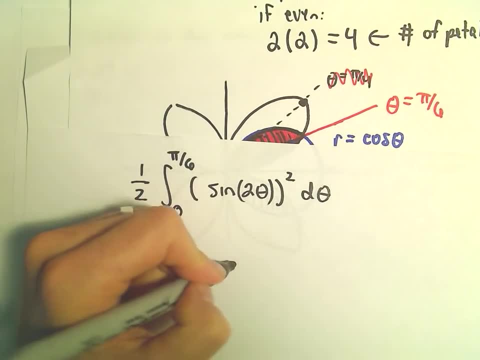 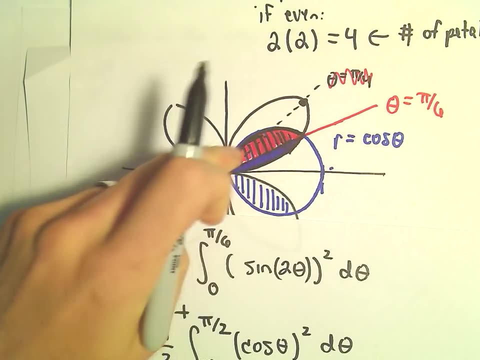 The region's bounded by the circle which is cosine theta. So we're going to have cosine theta quantity squared d theta And again that's only going to give us the top part. So what we're going to do to get the entire shaded area? 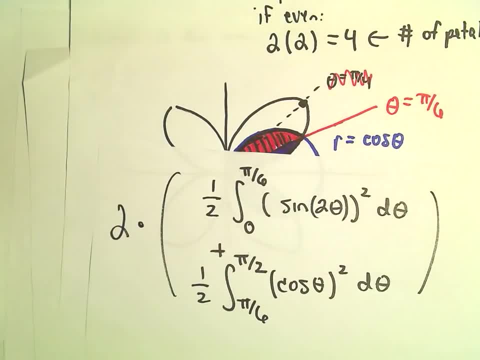 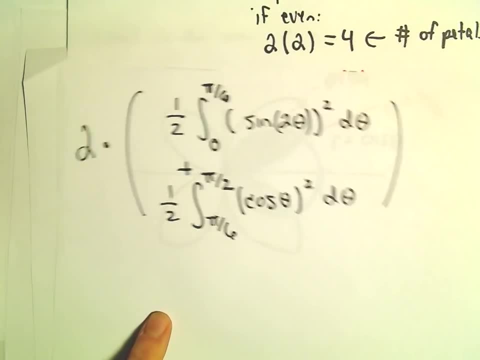 is, we'll take all of this and we'll multiply it by 2. All right, that's kind of the first step of this, I think, is just getting it set up. I think this can all be definitely a good bit confusing. 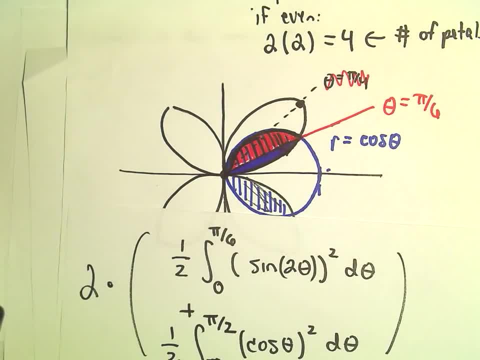 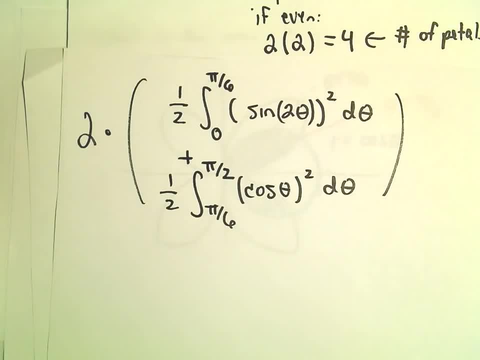 So again, you know just kind of. I think sketching the curves will help a lot, So hopefully that part makes sense. Let's now actually talk about computing these lovely integrals. So what we'll have to do is use a couple identities. 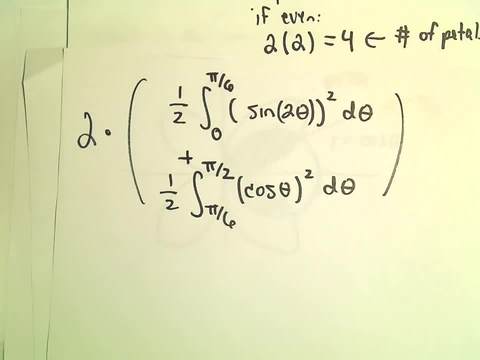 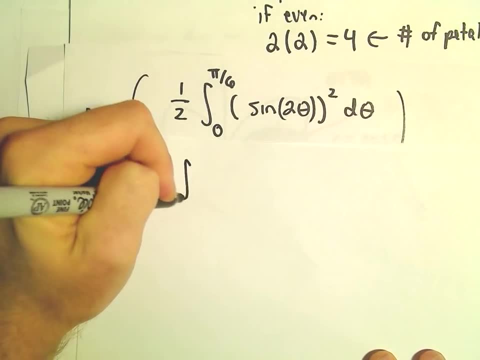 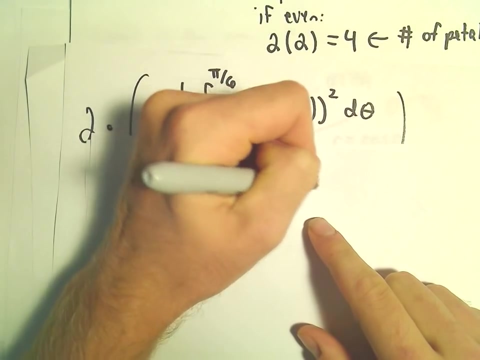 So let me compute. I'm just going to compute this integral from 0 to pi over 6 of sine squared 2 theta. Well, again, this is where we'll have to use our identity: 0 to pi over 6.. 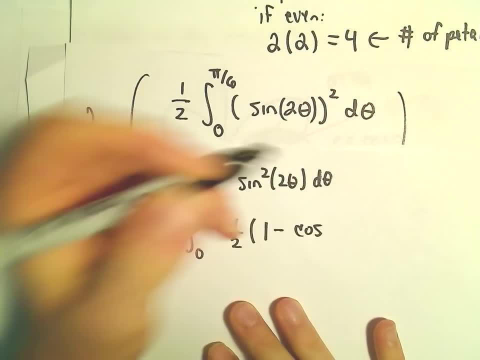 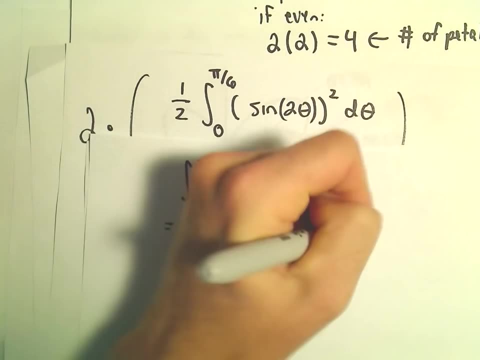 So this is going to be 1 half 1 minus cosine Again. whatever's on the inside, we double that. So instead of 2 theta we're going to get 4 theta d theta. So let's see we can pull the 1 half out front. 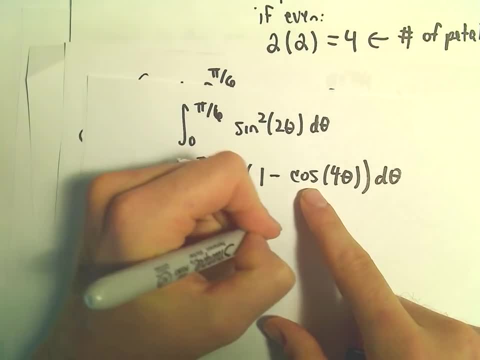 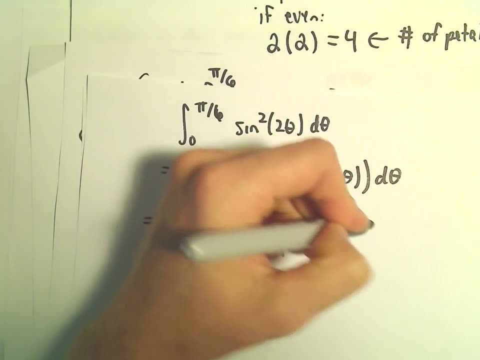 We can integrate this. This is going to be theta. We'll get minus sine of 4 theta over 4.. Again, we'll evaluate that from 0 to pi over 6.. So let's see here We'll get 1 half theta. 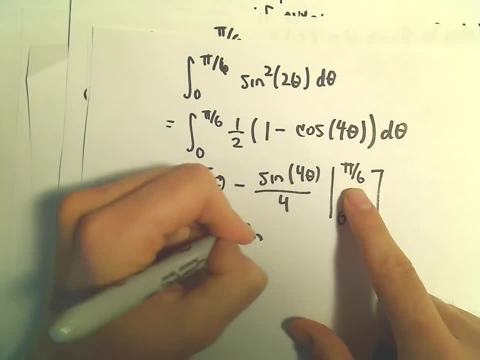 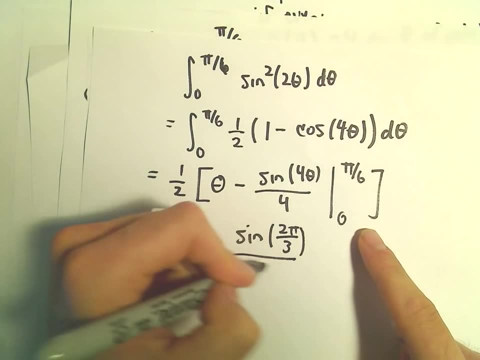 Again it's going to be pi over 6, plus sine of 4 times pi over 6 is going to be. I guess that will reduce to 2 pi over 3, all over 4.. And then we've got to subtract away our lower limits. 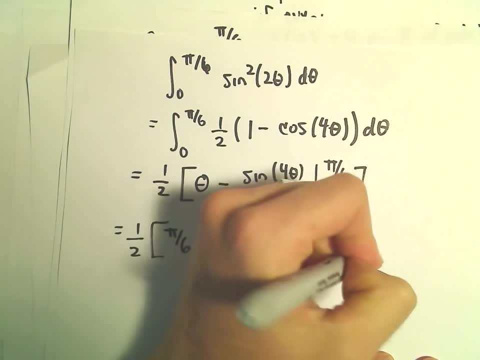 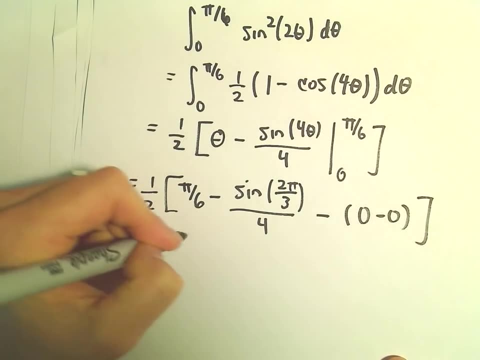 So when we plug in 0, we'll get 0 and sine of 0, which is also 0. So it looks like we're left with 1 half times pi over 6, minus. well, let's see sine of 2 pi over 3.. 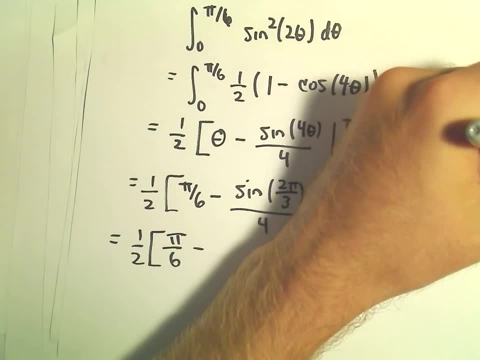 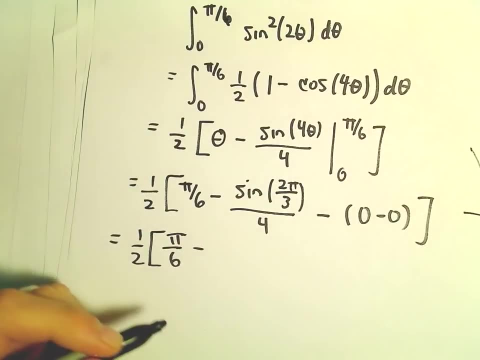 I always have to stop and think about these. Sine of pi over 3,, I guess, is going to be root 3 over 2.. So sine of 2 pi over 3 should also be root 3 over 2.. 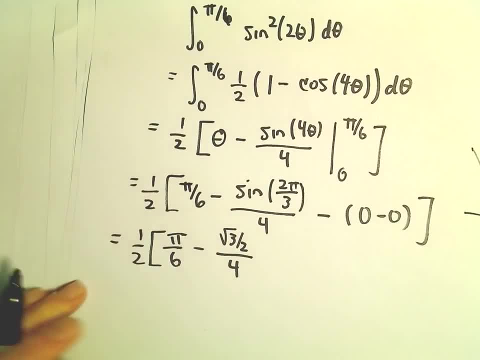 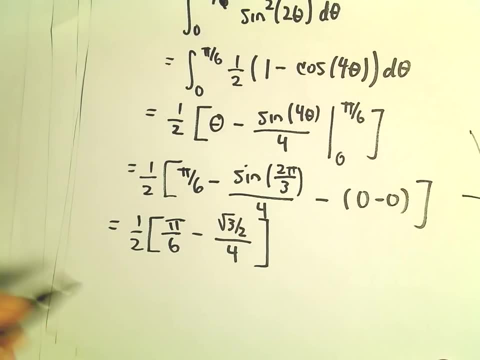 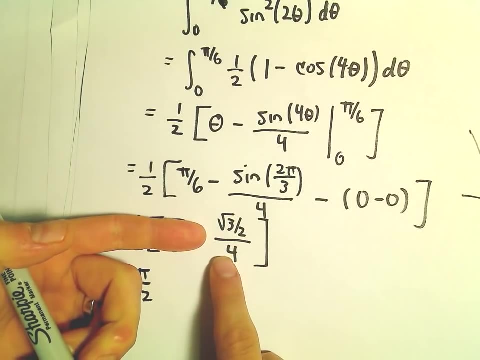 So we'll have square root of 3 over 2, all over 4. And then we'll subtract away just 0.. So let's see, This is going to give us pi over 12.. This part we would have 3 over 2 times 1. fourth: 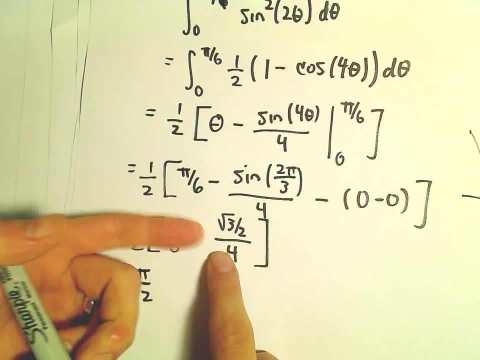 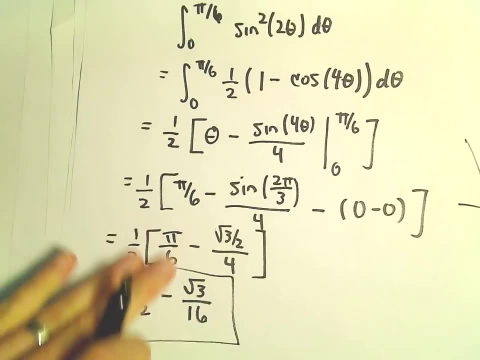 equivalently dividing by 4.. So that's going to give us root 3 over 8.. But when we distribute the half we'll get root 3 over 16.. All right, So that will be useful. And notice again, I didn't even multiply this by the half. 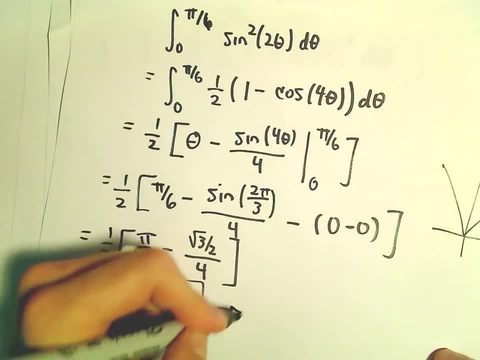 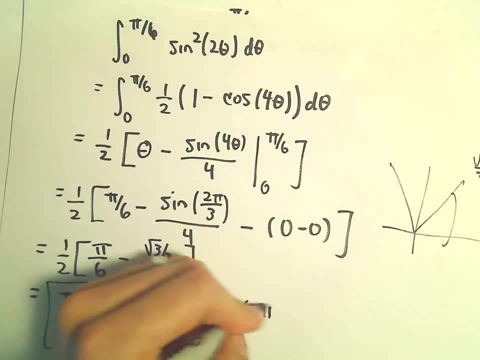 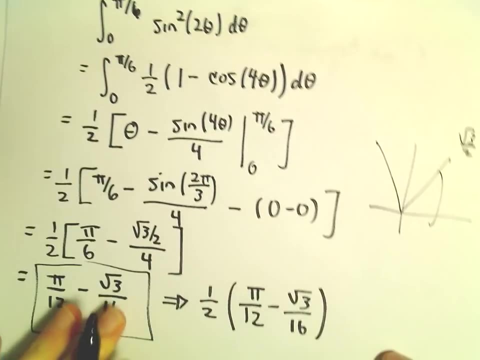 So I just computed the integral. So if we take 1 half of the integral, 1 half of the integral from 0 to pi over 6, we'll have to take 1 half of this stuff. Just a lot of bookkeeping here now. 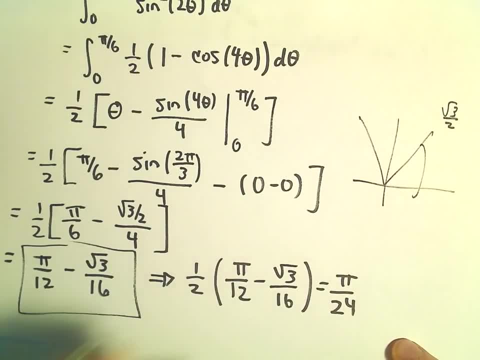 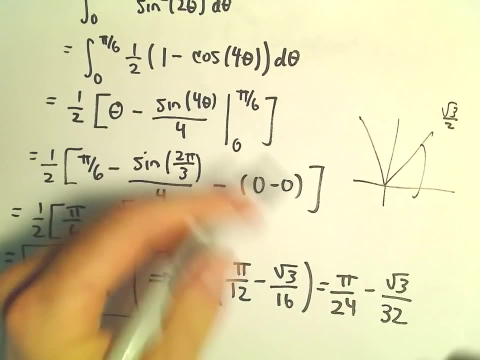 This is going to give us pi over 24,, I guess, minus the square root of 3 over 32.. Again, there was a 1 half that appeared, but that was just simply from the trig identity, So that's going to be important. 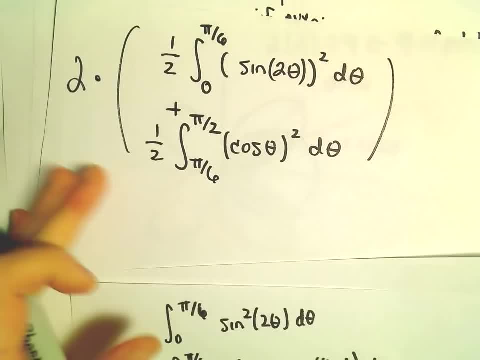 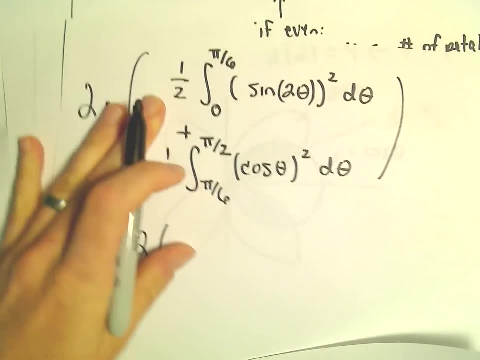 That will be the value for the top integral. So it says again we're going to get 2 plus the first integral, so 1 half times the integral from 0 to pi over 6, sine of 2 theta squared. 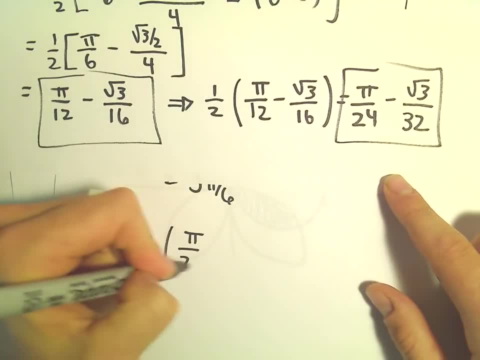 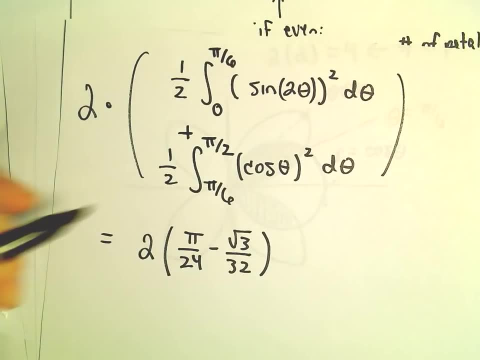 That's what we just computed. That's going to be pi over 24 minus the square root of 3 over 32.. So it says we get 2 times. we get that integral plus. we'll have to evaluate the other one as well. 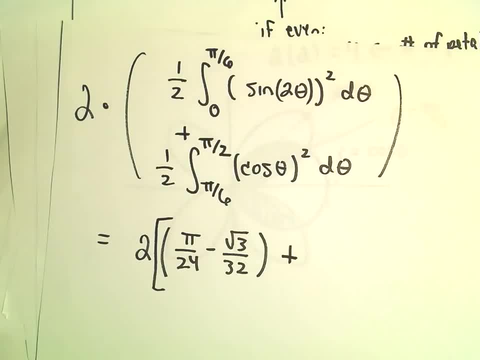 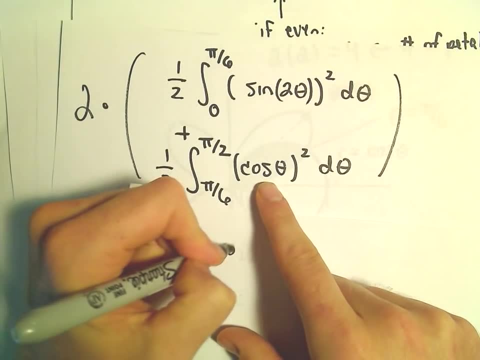 So let me do that now. So now I'm going to compute the integral from pi over 6 to pi over 2.. This is just going to be cosine squared theta. Again, we'll have to use our trig identity on the second one. 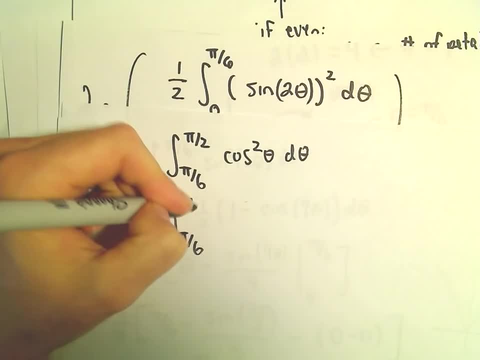 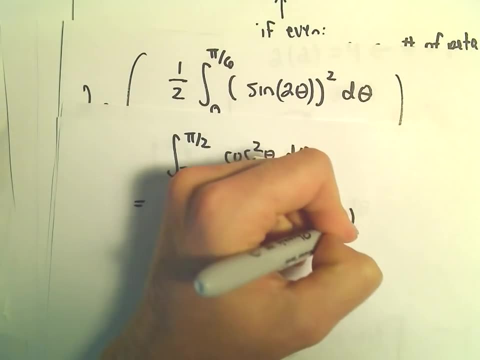 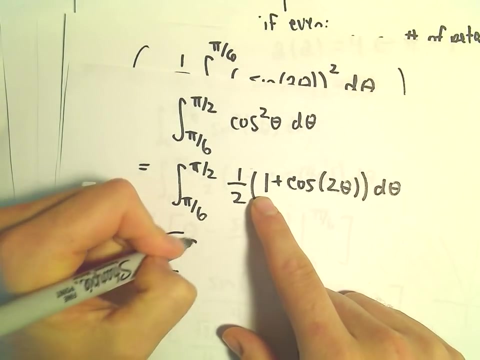 So let's see, pi over 6 to pi over 2, this is going to be 1 half, 1 plus cosine of 2, theta d theta. So let's see, we've got 1 half. the antiderivative of 1 will just be theta. 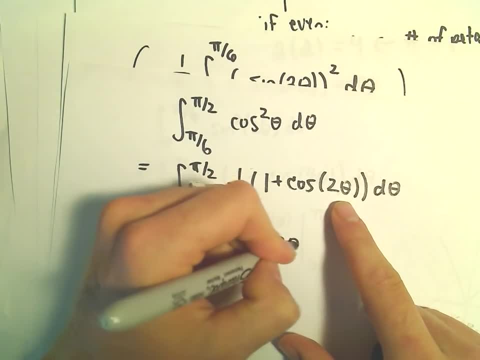 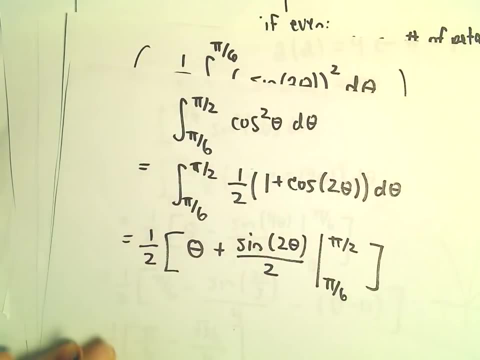 and then we'll have, plus sine 2, theta all over 2.. Again, we'll evaluate this from pi over 6 to pi over 2.. All right, so we're going to get 1 half times. we'll plug in pi over 2.. 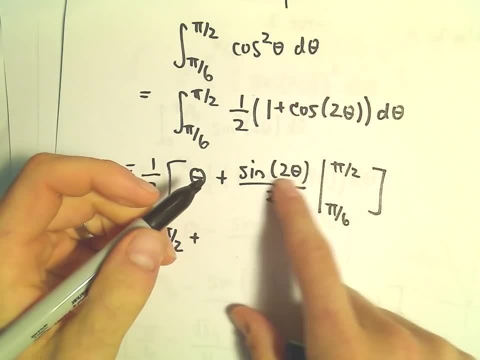 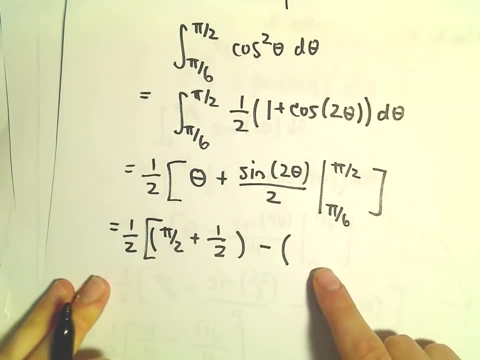 We'll get sine of 2 times pi over 2, which is going to be sine of pi. Sine of pi is 1, so we'll be left with 1 half minus the lower limit of integration. We'll plug in pi over 6.. 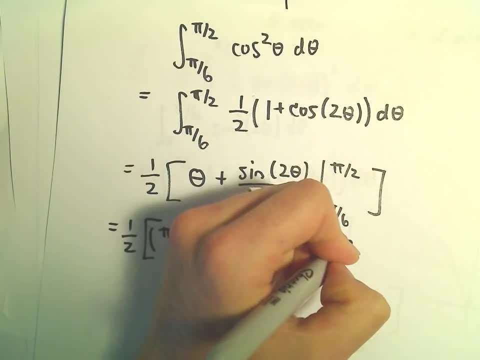 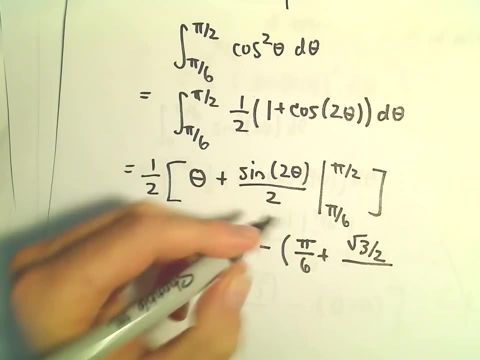 And then we'll get sine of 2 times pi over 6, which is going to be sine of pi over 3.. Well, let's see, we just said sine of pi over 3 is going to be root 3 over 2.. 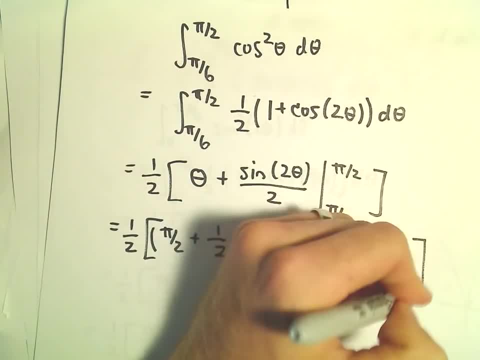 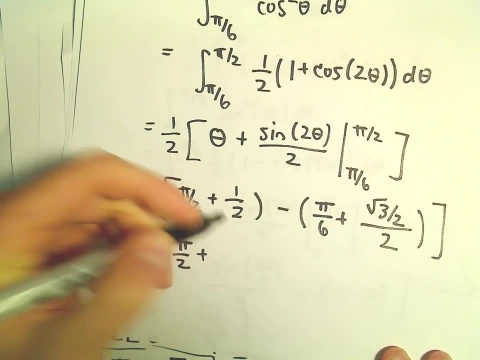 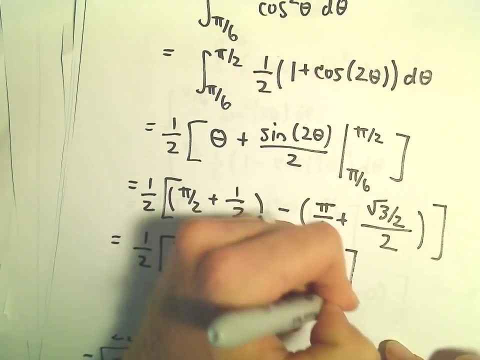 Again all divided by 2.. All right, so what do we have here? We've got 1 half times pi over 2, plus 1 half minus pi over 6. minus this will be square root of 3 over 4.. 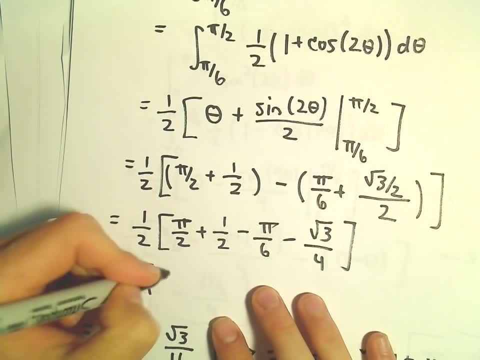 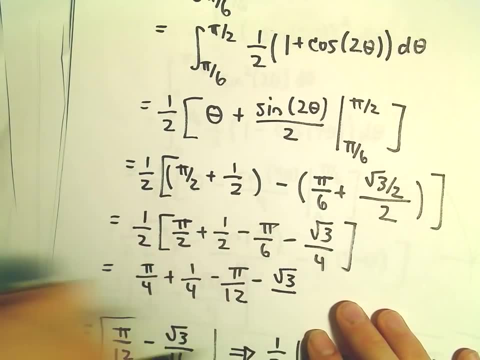 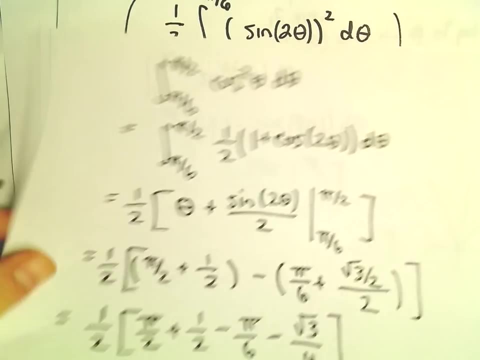 So again, we can always multiply this by 1 half. We'll get pi over 4 plus 1 fourth minus pi over 12, minus the square root of 3 over 8.. Let's see, so that's going to be the value of our integral. 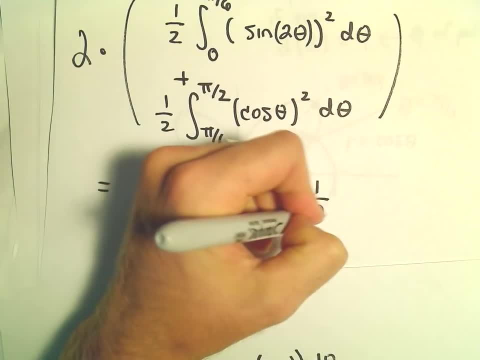 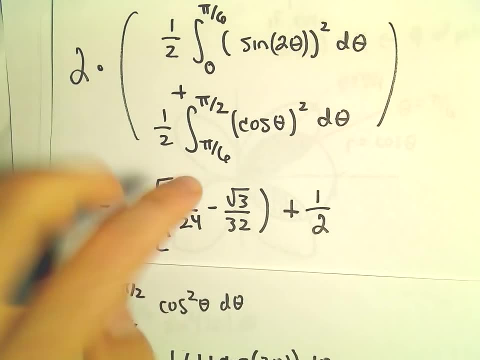 But again we have to multiply that by 1 half as well. I should have just distributed the 2 at the beginning right and got rid of it, but whatever. So we have 1 half times the integral from pi over 6. 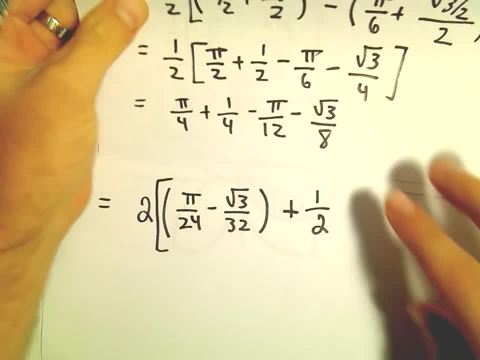 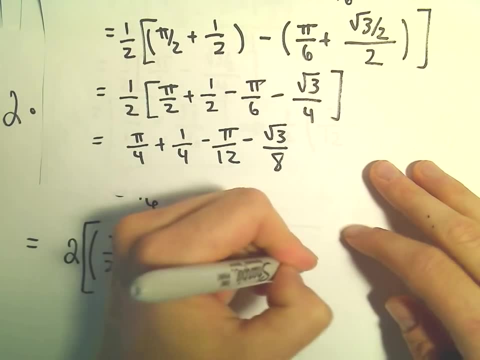 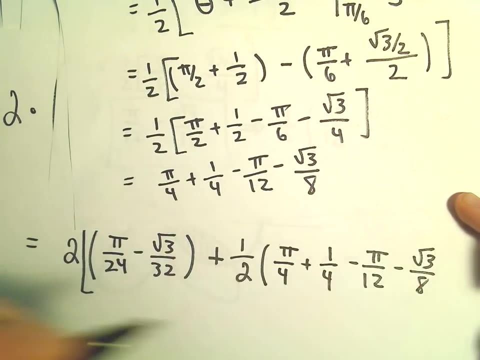 to pi over 2 of cosine squared Again, that's where we're getting this value: pi over 4 plus 1, fourth minus pi over 12, minus the square root of 3 over 8.. All right, so here, if we distribute the 2,, 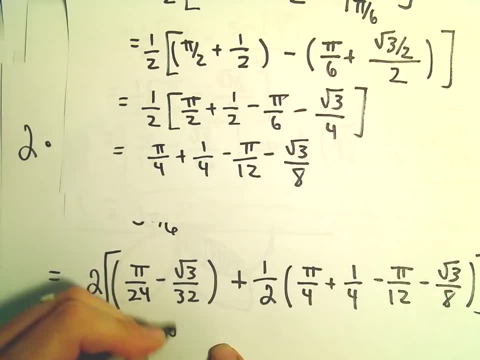 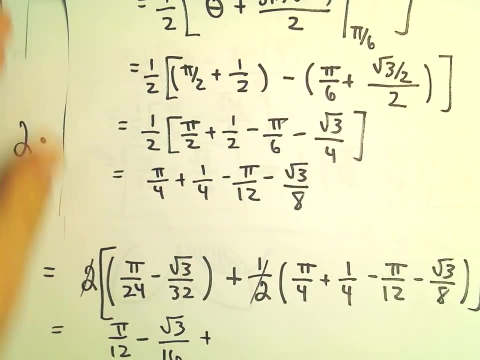 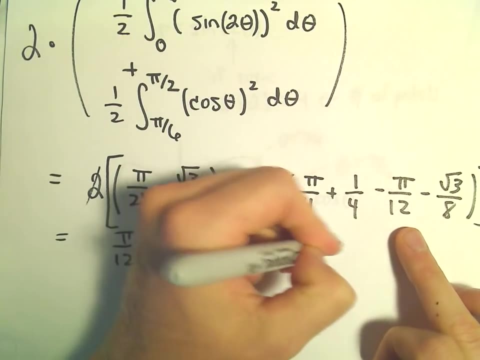 we'll get pi over 12 minus square root of 3 over 16.. The 2 times the half would just cancel. So then we would be left with pi over 4 plus 1 fourth minus pi over 12, minus square root of 3 over 8.. 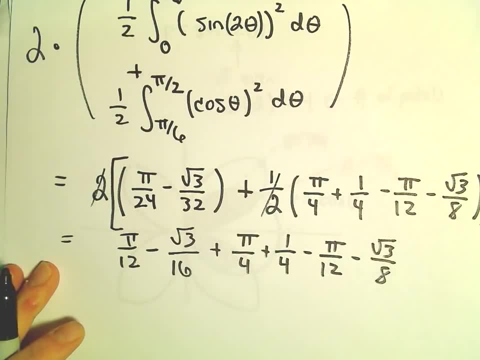 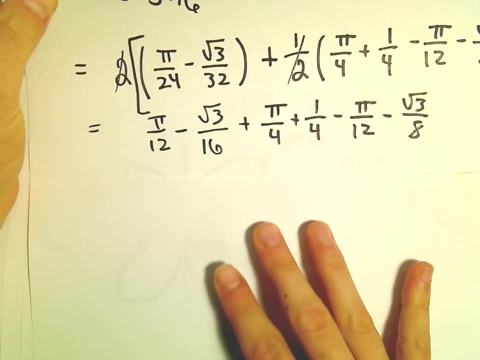 And, of course, you could always start getting common denominators and simplifying this a little bit more. I guess let's go ahead and do that. We're so close, Grab one more piece of paper, All right, so we can always combine this a little bit more, I guess.